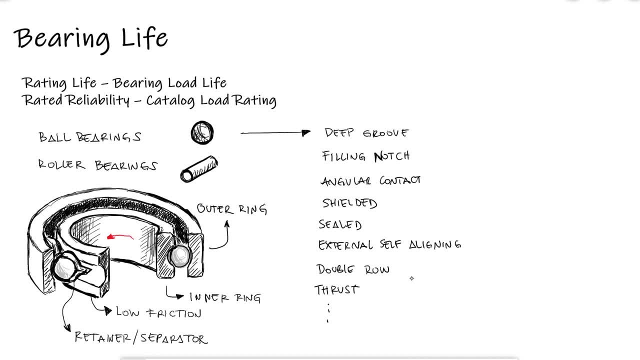 the radial loads. You can easily do that by checking the manufacturer's datasheet of the part you're looking up. As you would imagine, if any foreign material, like dirt, comes into the rolling elements, it will be bad for the bearings. so you might want to consider within that wide range of 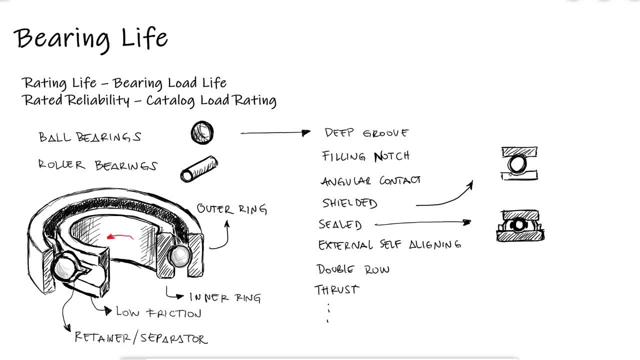 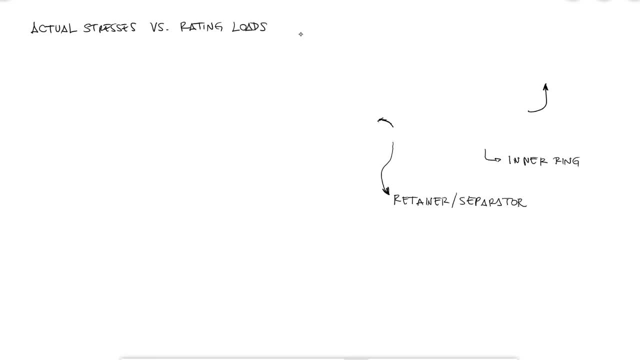 different types of bearings to select one that is sealed or that has a shield on at least one side. When bearings are under service, contact stresses occur on all three main elements: the inner ring, the balls or rollers, and the outer ring, The curvature of the surface in 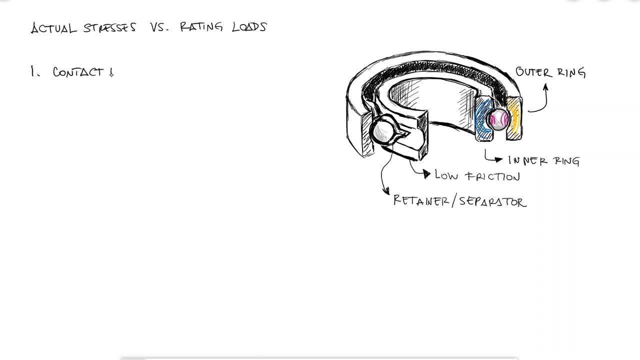 contact is not as simple as a cylinder and cylinder, like with pitting of gears or even a cylinder on a cylinder. Think, for example, of the contact between the ball and the outer ring. The curvature of the outer ring, which would be a cylinder, is oriented in the same direction as 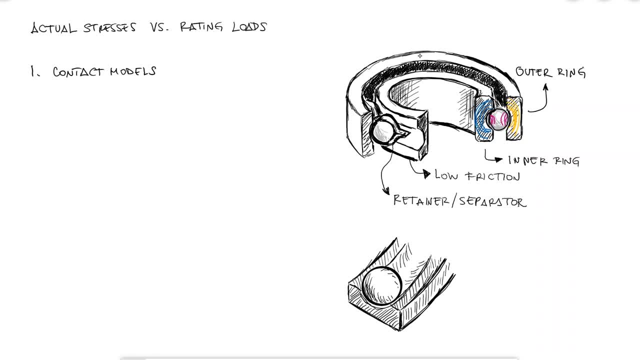 that of the ball. It would be a sphere on the inner surface of a cylinder, a concave surface which is both concave to match the ball, but also concave in the tangential direction, as it is still a ring. For this reason, more complex equations are needed than those that 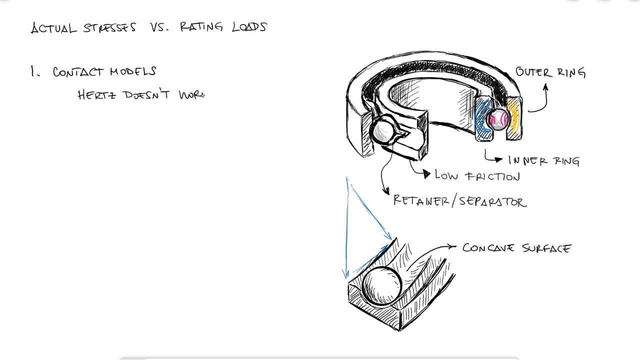 the Hertz contact model can offer even for more complex geometries. Additionally, the forces that push these components are not just only axial or only radial. The balls and rollers will be pushed towards edges and other more irregular geometries inside the bearing, even the separators I mentioned before. More importantly, even when you 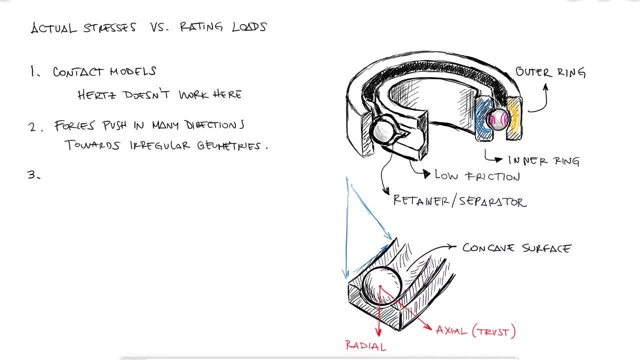 find a good equation or model that allows you to calculate the stresses. they would only hold for when the bearing is clean, properly lubricated, sealed against dust and dirt, perfectly mounted, operated at a stable and reasonable temperature, etc. For these three reasons mainly, we use a bearing life to refer to the number of revolutions of the. 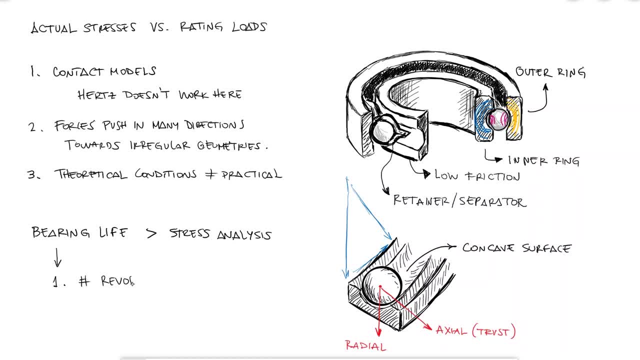 inner ring until there's signs of fatigue, as opposed to trying to calculate the actual stresses. Alternatively, we can also use bearing life to refer to the number of hours for a specific rotation speed, which obviously ends up being the same thing. This sign of fatigue has been. 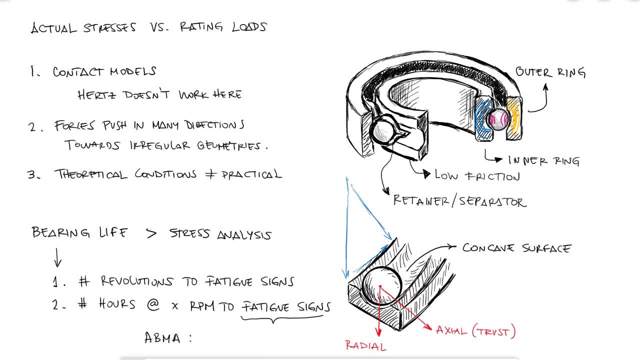 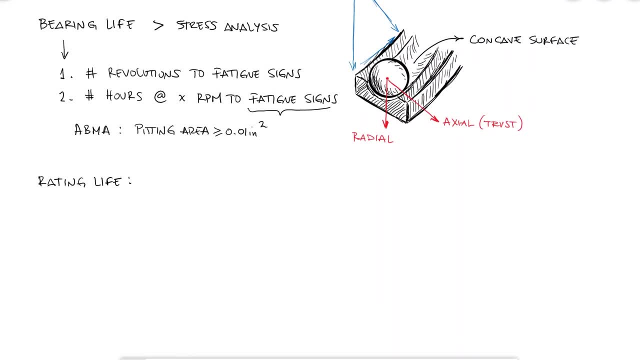 defined by the American Bearing Manufacturers Association as a pitting area of 0.01 inches squared. The rating life is the number of revolutions, or again, the hours at a constant speed for which 90% of a group of bearings being tested will not show failure signs. 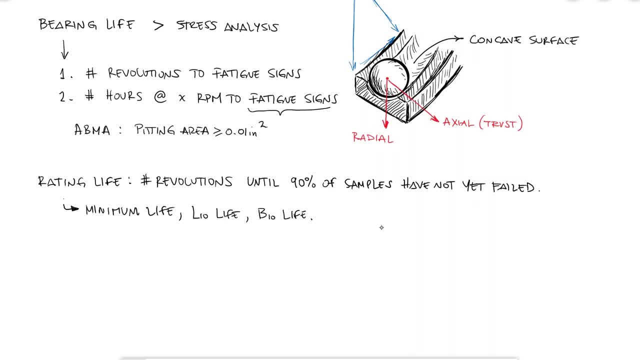 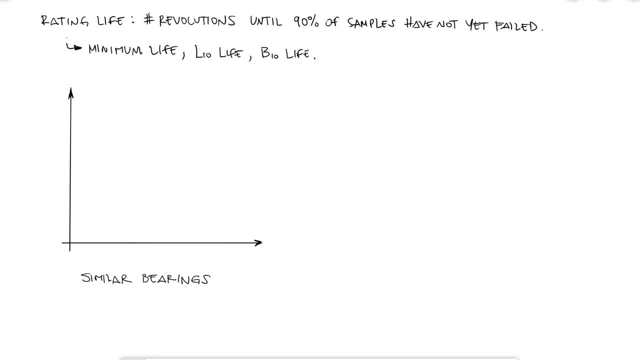 Minimum life, l-10 life and b-10 life are also used to refer to this rating When similar bearings or bearings of the same category and type are tested in a lab. you see that when plotting the load versus the rating life. 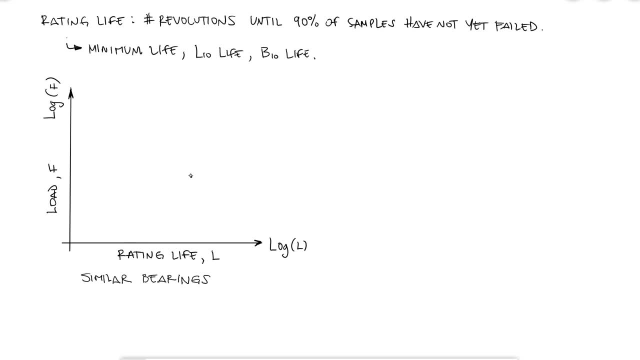 on a log-log plot: for the smaller loads, the rating life will be longer, and for the higher loads, the rating life will be shorter, and all the results land on roughly the same straight line. Now we've done this analysis many times before, for example, the ultimate strength for spring wires. 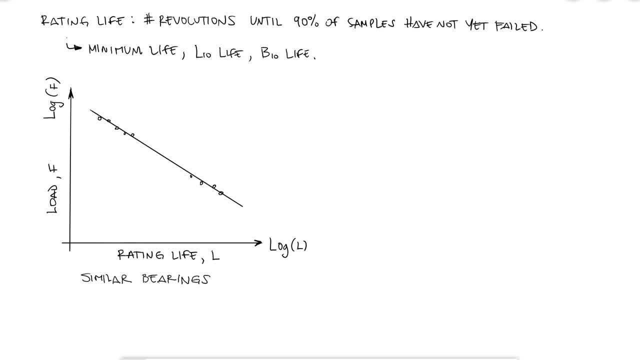 link below where we found the equation of a straight line on a log-log plot. The equation of the straight line with a negative slope looks like y equal to a constant, over x to an exponent, and this is without the logarithms. y would be the force, x is the rating life L. 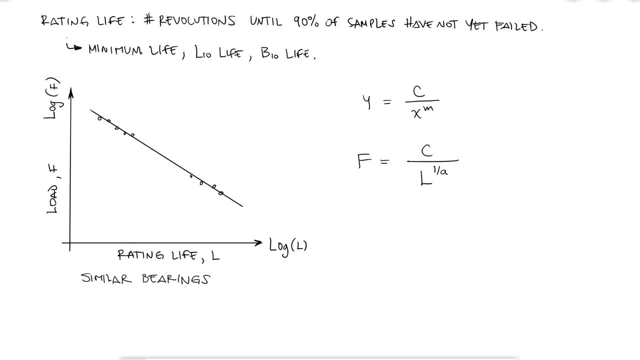 and we can write the exponent as 1 over a. This means that f times L to the 1 over a is constant. Experimentally we learned that a takes a value of 3 for ball bearings and 10 over 3 for roller bearings, tapered or cylindrical roller. What the manufacturers will report. 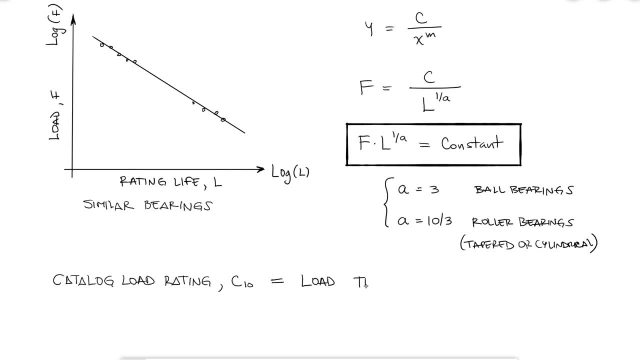 is the catalog load rating C10,, which is the radial load that causes failure. Now, remember that this load is the one that will cause 10% of the samples to fail, So this intrinsically already has a rated reliability of 90%. 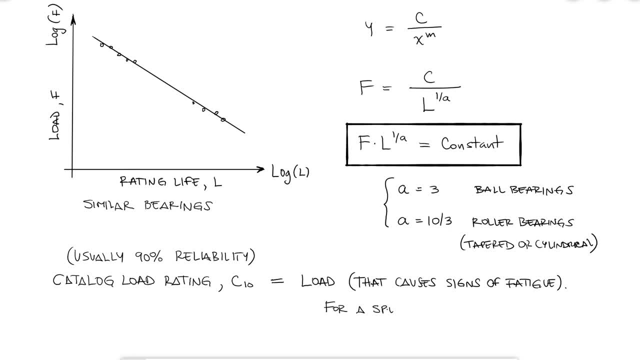 The other thing that the manufacturer will have to report is the number of cycles they used for testing, Since 10 to the 6th is not a lot for bearings. a huge force would have to be used for them to fail that quickly. So this number is usually more than 10 to the 6th, although a 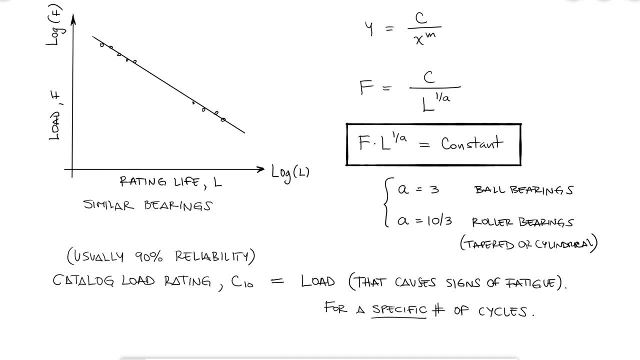 couple manufacturers still use this number. Regardless. this is all the info we need. If we know the force that our specific application will cause on the bearing and the life equation, then we know that the number of cycles they used for testing is not a lot for bearings. So this intrinsically already has a rated reliability of 90%. So this number is usually more than 10 to the 6th, although a couple manufacturers still use this number. Regardless, this is all the info we need If we know the force that our specific application will cause on the bearing and the life equation. 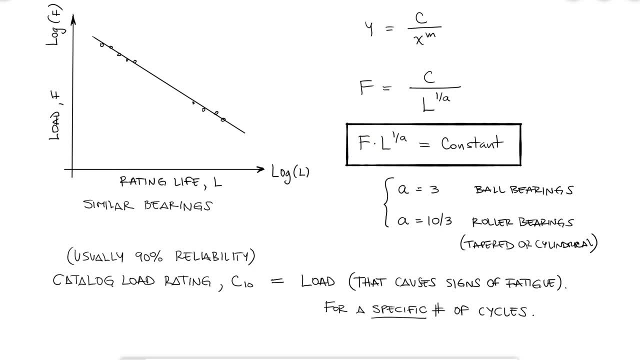 We know that the force that our specific application will cause on the bearing and the life equation expectancy we would like the bearing to have and we know that the value of F times L to the 1 over A is constant. then we can use a manufacturer's catalog and their life rating information. 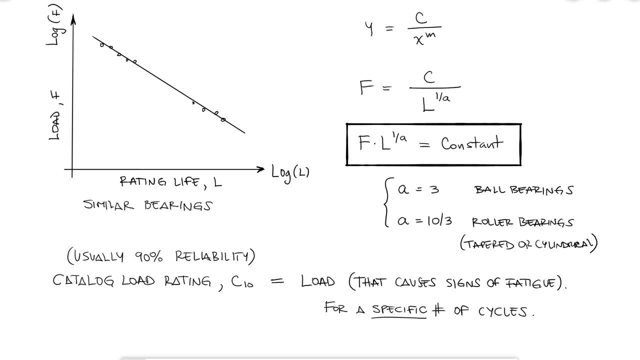 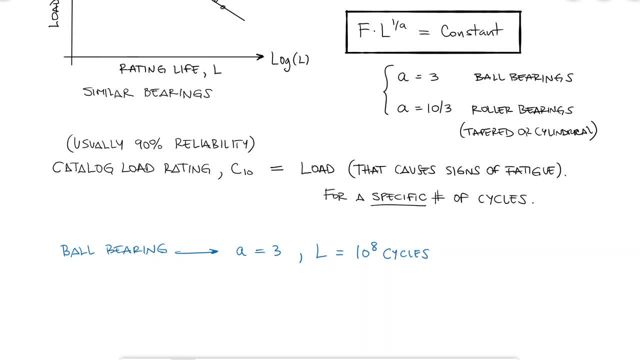 to select a gear that will have the same F times L to the 1 over A value, For example, if I want my ball bearing to last 100 million cycles and I know that the radial force going into the bearing is 400 pounds. 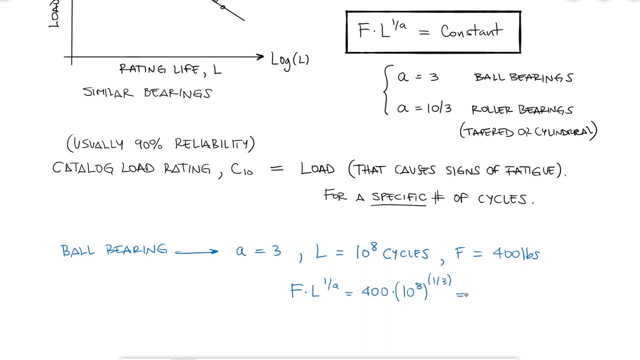 the constant in this case would be a little over 185,000.. If a manufacturer rates its bearings for a life of 1 million cycles, I would need to find a bearing that is rated for a force that, when multiplied by L to the 1 over 3, or 10 to the 6th to the 1 over 3, gives me a value. 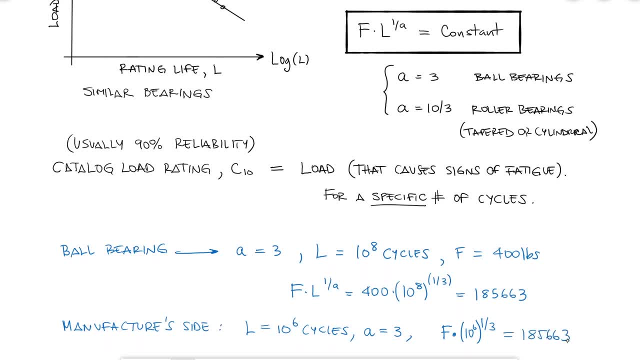 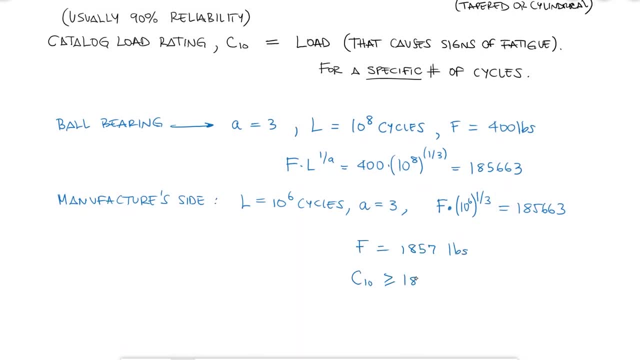 of 185,000,. since that value has to be constant, That would be in this case a catalog load rating C10 of 1857 pounds or higher. We usually use a capital R subscript for rated and a capital D. 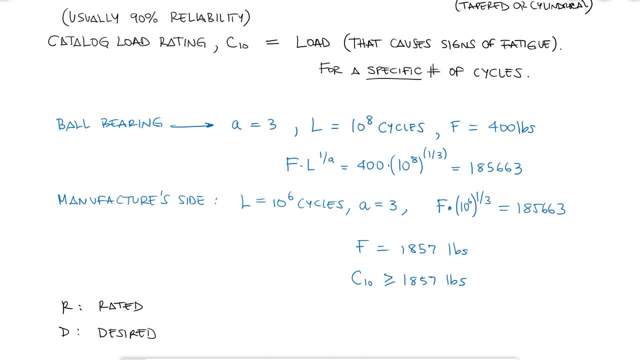 subscript for desired. This means that the expression we use to find an appropriate bearing for our particular application would be FR times LR to the 1 over A, equal to FD times LD to the 1 over A, Since the rated force is what we know as the catalog load rating C10, just remember that. 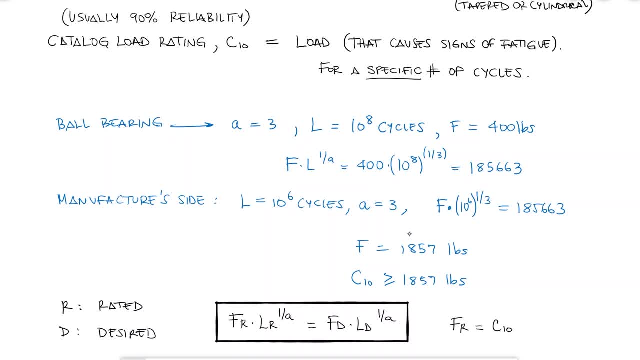 FR is equal to C10.. Of course, since some manufacturers use the rating life in hours for a specific rating speed, which is usually in revs per minute, instead of using the rating life in hours for a specific rating speed, which is usually in revs per minute, 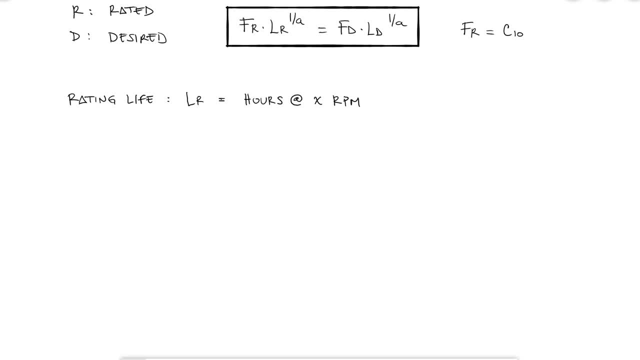 instead of using the number of revolutions to failure, you would then need to carry out an extra step of translating the number of cycles for that specific time and speed. Time in hours times. rotation. speed in revs per minute times 60 minutes in one hour would give you the total. 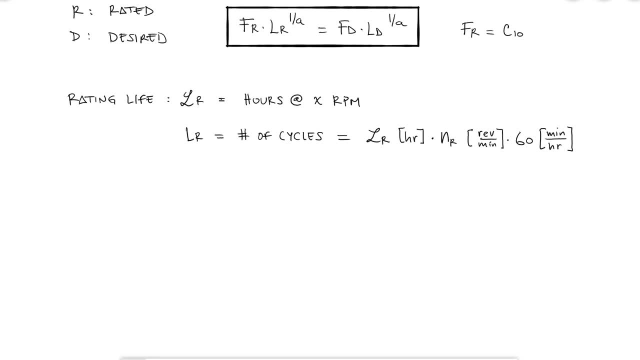 number of revolutions. Let's solve a simple example where the manufacturer SKF, a popular Swedish bearing company, rates its bearings for 10 to the 6th cycles. We've calculated all of the interaction forces between two spur gears and with them we can calculate the number of. 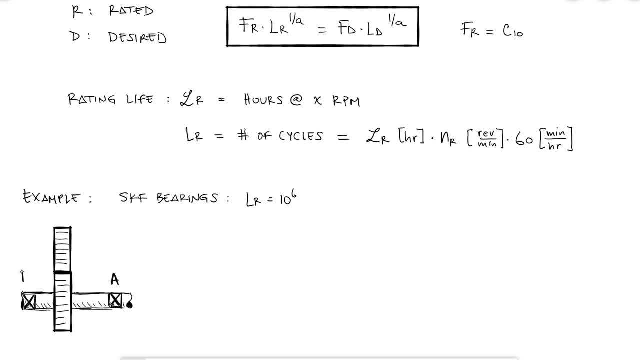 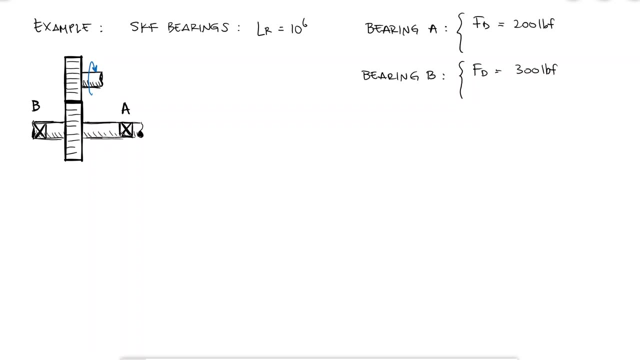 reaction forces at the bearings. following the procedures we learned and followed during past videos- links below- We know that the radial load that bearing A will be subjected to is 200 pounds and 300 pounds for bearing B. If we know that our gear shaft bearing system needs to be running for. 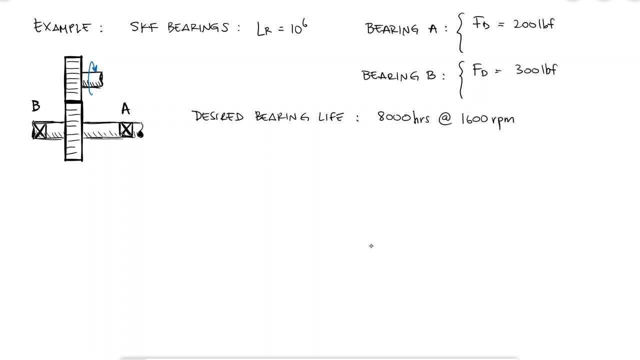 8,000 hours at 1,600 RPM. what is the catalog load rating- C10- that I would choose for each roller bearing for a 90% reliability To solve this problem? I know that the procedure is going to be the same for bearing A and bearing B, If I know the desired load that. 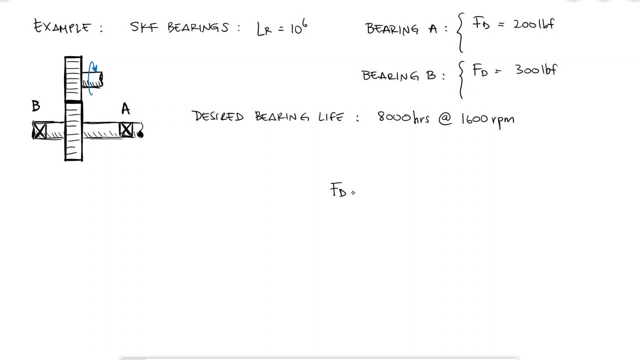 bearing A or bearing B are supposed to withstand and the number of cycles that they're supposed to withstand- and I know that the bearing company rates its bearings for a rating life of 10 to the 6th cycles- I can easily solve for C10. The desired number of cycles for bearing A and B. 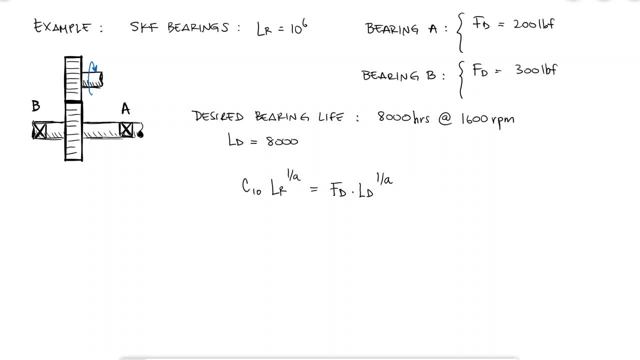 is going to be the same and it would be equal to 8,000 hours times 1,600 RPM times 16 minutes in every hour. Since the procedure is going to be the same for bearing A and bearing B, if the question is asking for the C10 of a roller bearing, I know that A is equal to 10 over 3.. 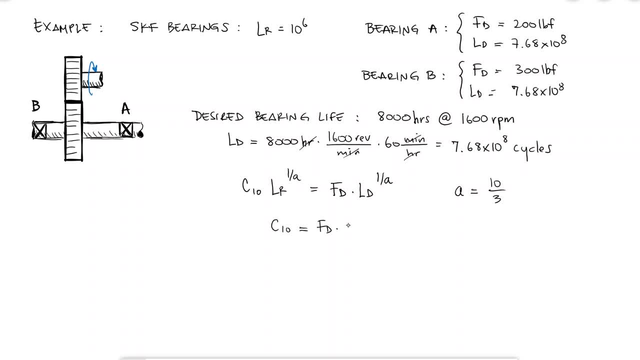 The catalog load rating C10 can then be solved for, in terms of the other variables, FD would be 200 pounds for bearing A and 300 pounds for bearing B. This tells me that I need a catalog load rating higher than 1,468 pounds for bearing A and a catalog load rating higher than 2,202 pounds. 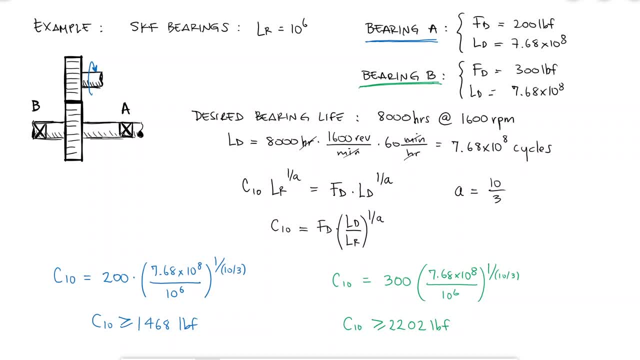 for bearing B, And if the manufacturer uses the C10 for bearing A and bearing B, then the C10 is going to be the same for bearing A and bearing B. If the manufacturer uses metric units, which is very common around the world, I can just convert the units of my answer. 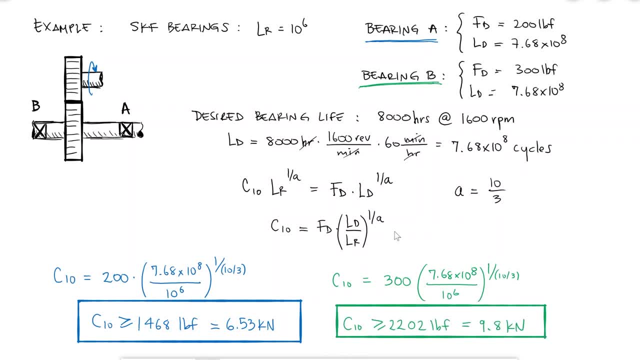 There's one more example like this in the description below, if you want to check it out. Notice that these values correspond to a 90% reliability, which is what most manufacturers use anyways. However, for certain applications, I would probably not want to risk fatigue signs. 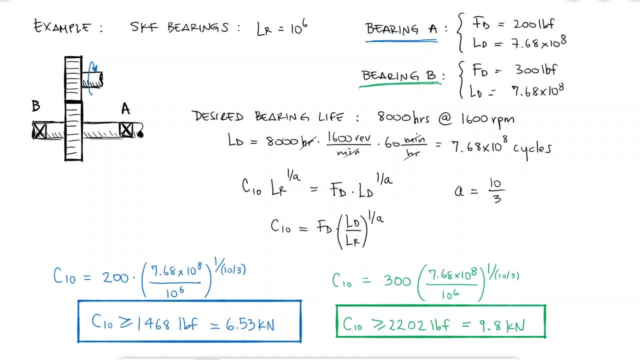 in the bearings that could potentially ruin my machine, with a 10% chance of it happening. In the next video we will talk about reliability and how to calculate the catalog load rating with a reliability other than what the manufacturer lists or uses for its experiments. 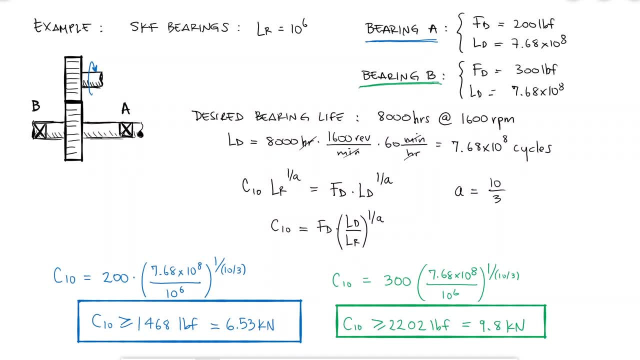 We will later introduce the concept of combined radial and thrust loading, since many applications, like we've already seen before, do introduce thrust to the shaft and therefore the bearing. Thanks for watching.